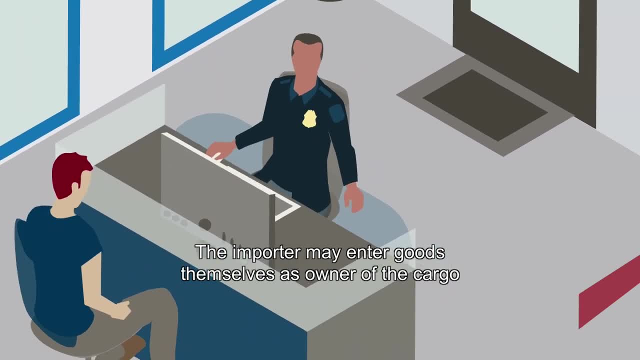 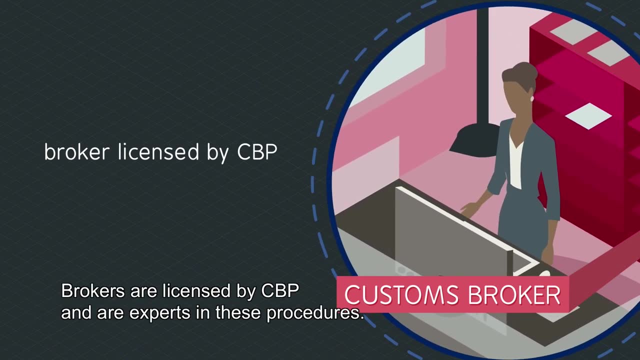 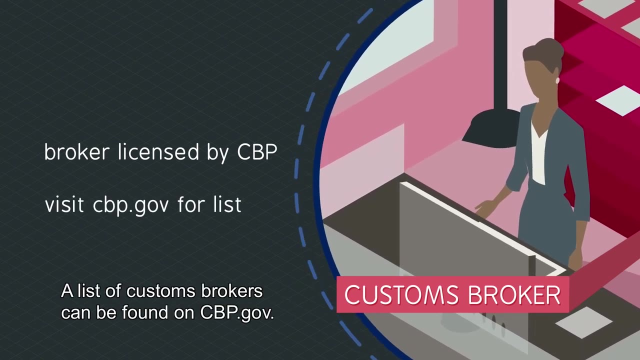 The importer may enter goods themselves as owner of the cargo or they may hire a customs broker As a shipper of goods. you may elect to have a broker. Brokers are licensed by CBP and are experts in these procedures. A list of customs brokers can be found on CBPgov. 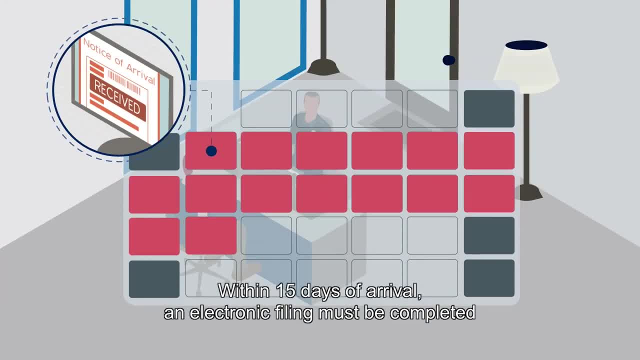 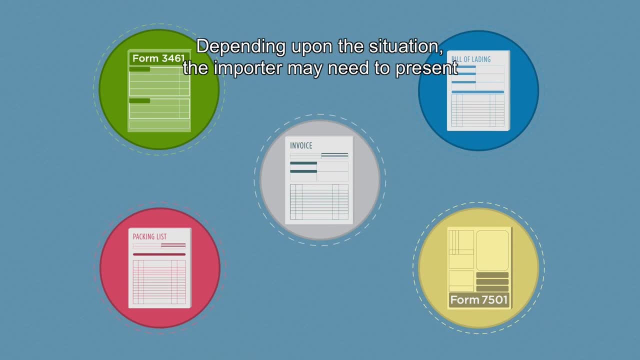 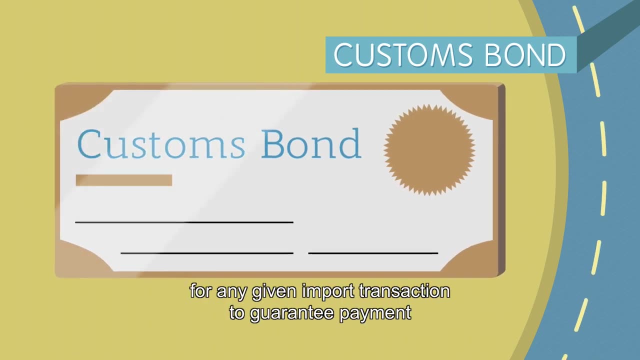 Within 15 days of arrival, an electronic filing must be completed on the Automated Commercial Environment, or ACE, system. Depending upon the situation, the importer may need to present other documents, such as a customs bond, which is a contract between customs and an importer for any given import transaction. 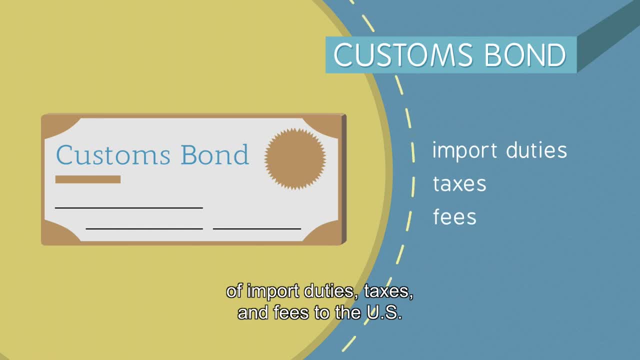 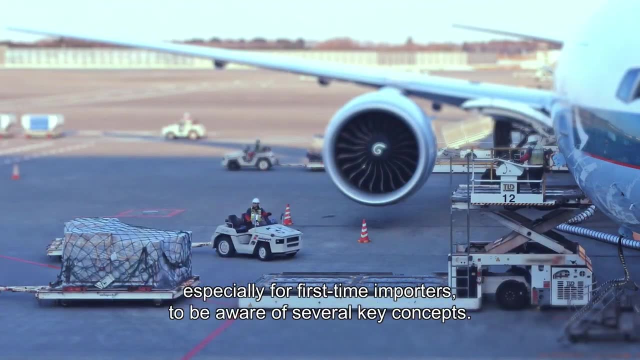 to guarantee payment of import duties, taxes and fees to the US. While there are different types of entries, it's important, especially for first-time importers, to be aware of several key concepts. Let's review some of them now. 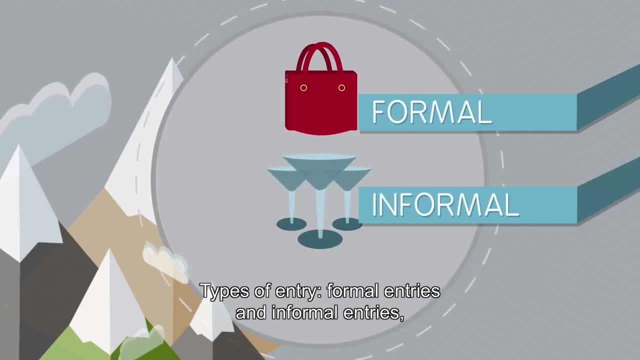 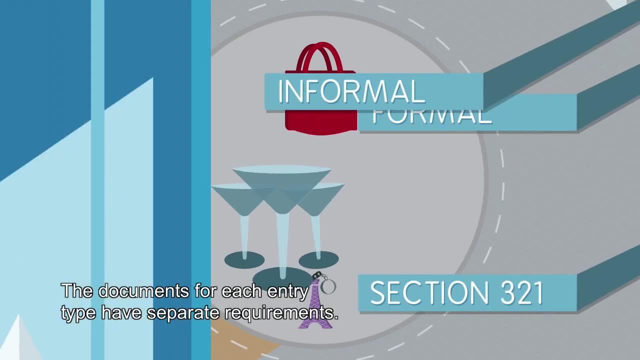 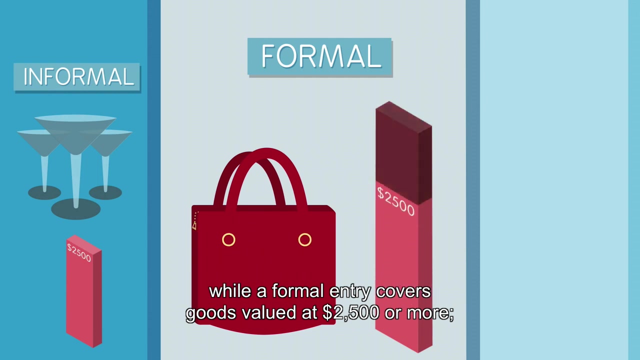 Types of entry: Formal entries and informal entries, including packages that qualify as Section 321- shipments. The documents for each entry type have separate requirements. An informal entry may involve goods valued less than $2,500,, while a formal entry covers goods valued at $2,500 or more. 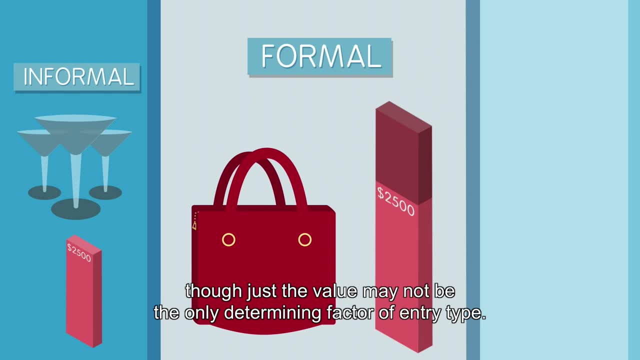 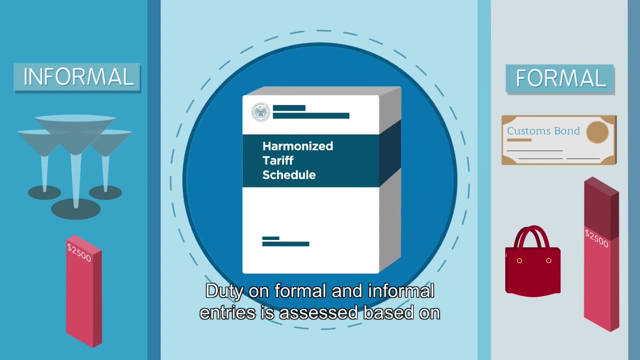 Though just the value may not be the only determining factor of entry type, formal entries also require formal entry. They require a customs bond. Duty on formal and informal entries is assessed based on how goods are categorized in the Harmonized Tariff Schedule of the US. 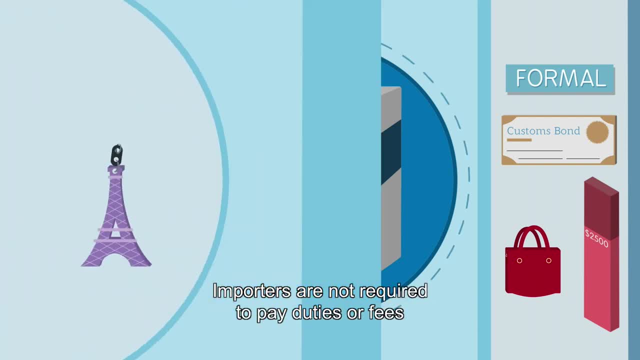 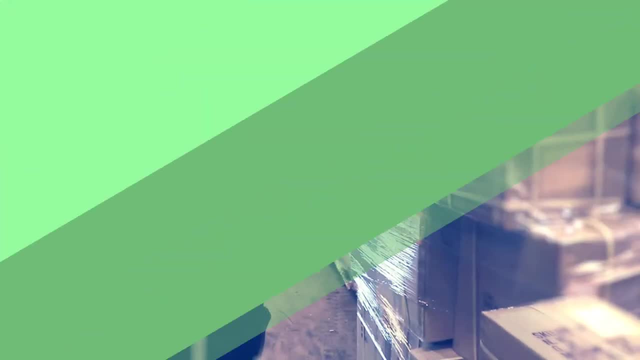 Other processing fees may be assessed as applicable. Importers are not required to pay duties or fees on goods less than $800 that qualify as Section 321.. If goods are selected for examination, CBP will inspect the shipment to determine if they're admissible. 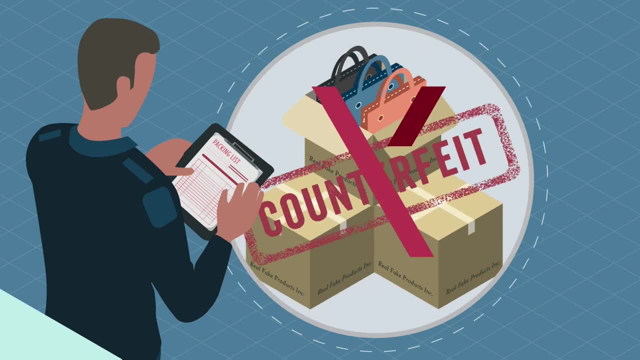 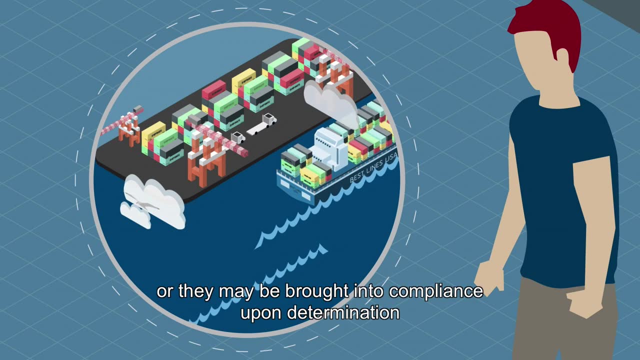 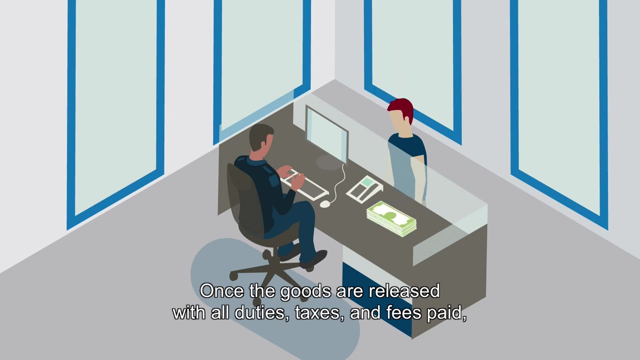 If applicable, they will be detained and may be seized. In some instances, importers may be permitted to re-export the goods or they may be brought into compliance upon determination that all import requirements have been ultimately satisfied, Once the goods are released, with all duties, taxes and fees paid.